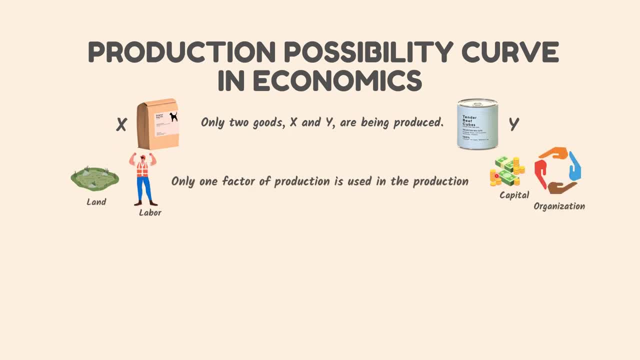 Number 2. Only one factor of production is used in the production. That factor of production is labor. The supply of labor in the economy is fixed and total amount of labor is 4%. That particular factory is fully employed. Number 3. The two goods can be produced in various ratios. This means that the country can produce more of X and less of Y, or less X and more of Y. 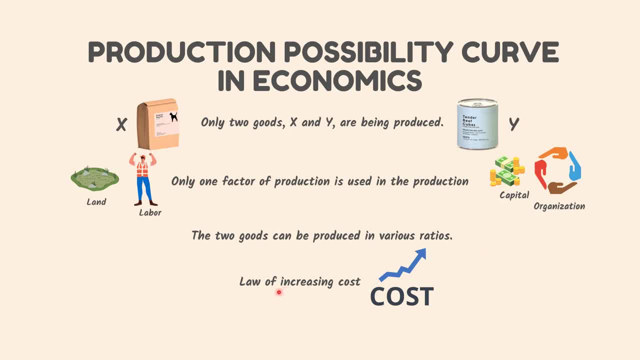 Number 4: In the production of both goods, law of increasing cost operates. This means that if the production of one good rises, its marginal cost will rise. Number 5. There is no change in production process or production technology. then explain how the production possibility curve can be obtained. 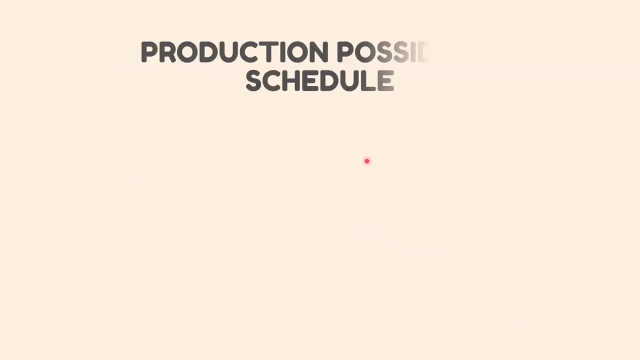 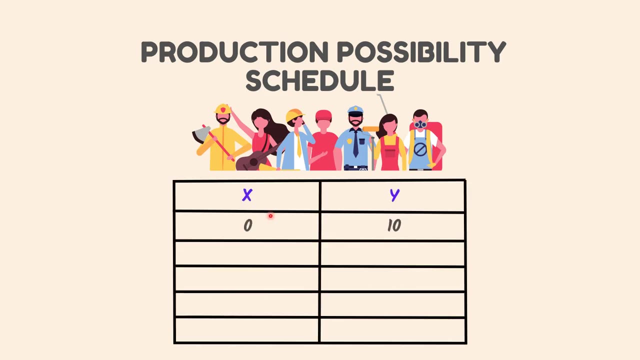 Suppose the country can produce different alternative combinations of X and Y with its given amount of labor. Those combinations are shown with the help of the following hypothetical schedule: When the country doesn't produce any X, then it can use all its resources to produce Y. 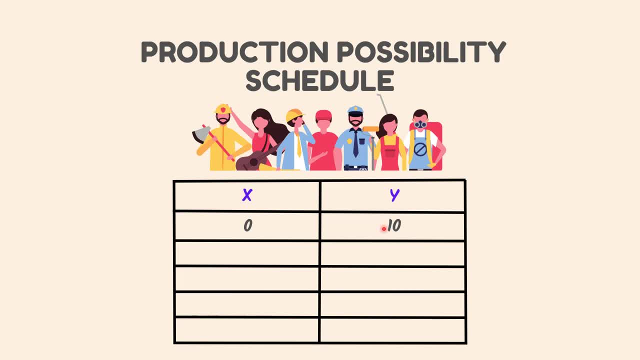 So Y is 10.. Now, if the country starts to produce the Xp1 unit, that will decrease the production of Y to 9.. When X is 2, the production of Y will decrease to 7.. Like this: when X is 3, Y is 4.. 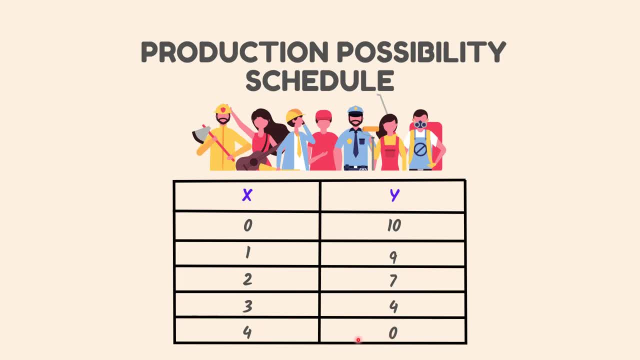 And at the last stage, when they use their all resource to produce 4 units of X, they can't produce any unit of Y. From this schedule we see that if the country produces only Y and no amount of good X, then it can produce a maximum of 10 units of Y. 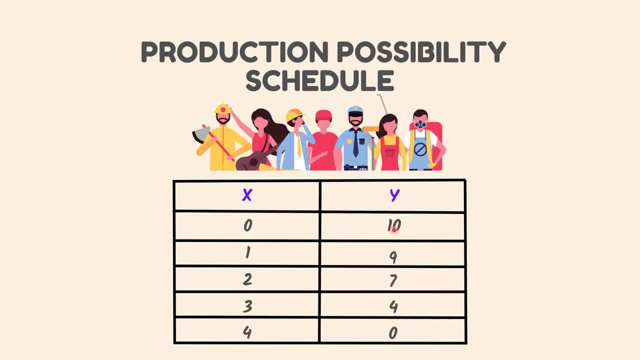 So we get a combination of 0 and 10. on the production possibility curve Again: if the country does not produce good Y and devote its entire resources in the production of X, then it can produce a maximum of 4 units of X. 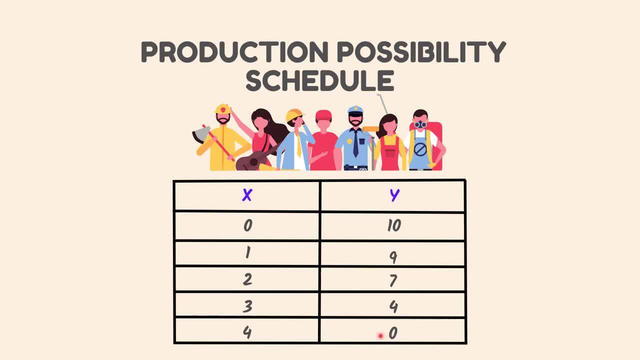 Hence 0.4 and 0 will be a combination of 2 goods on the production possibility curve. In this way, employing the entire resource labor, the country can produce 1 unit of good X and 9 units of good Y, or 2 units of good X and 7 units of good Y. In our figure we